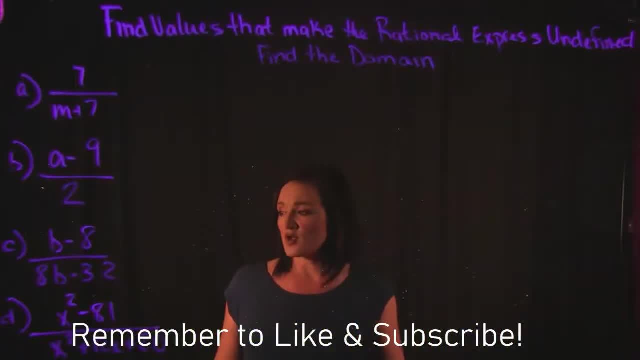 All right, guys. so for this particular video, we're going to work on four different examples, specifically finding the values that make the rational expressions undefined. And then we're going to go a step further and we're going to find the domain of these. So the following four: 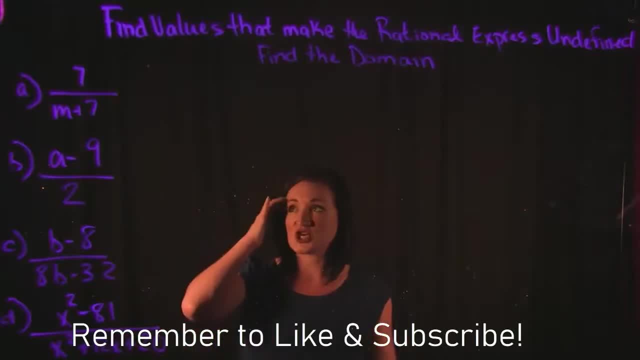 examples are all rational expressions. A rational expression is just where the numerator and denominator is a polynomial. So almost anything that you can write in fraction form is technically considered a rational expression. And because they're technically fractions, most people don't like fractions. A lot of people don't like necessarily dealing with these kind of problems. 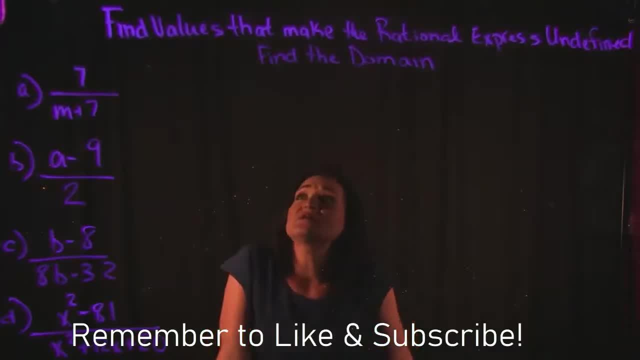 but let's try and make this a little bit easier here. So we want to specifically know what makes these undefined. Okay, so when you hear the word undefined, so a fraction is undefined when the denominator equals zero. So remember, you can't have a fraction where the denominator equals. 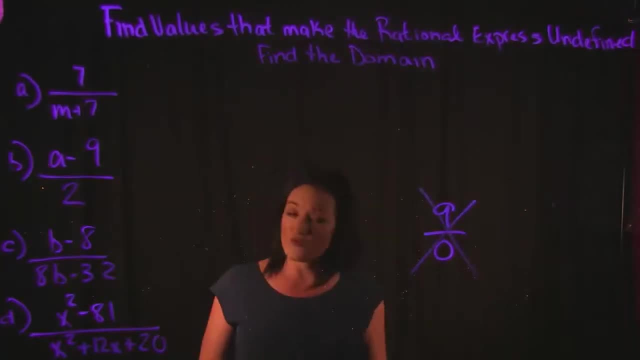 zero. When there's a zero in the denominator, it throws the whole fraction off. It's undefined. You just can't do it. You can't divide by zero. It makes no sense, It's just not allowable. So what we're trying to figure out is what. 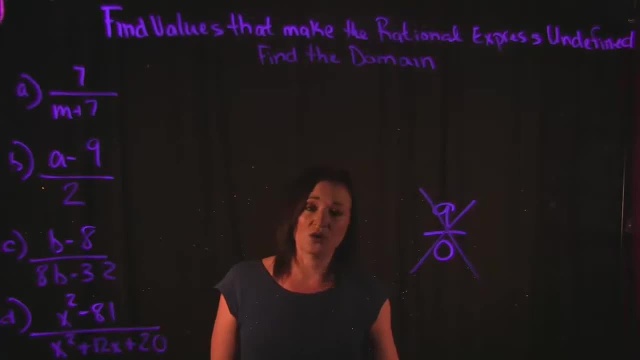 number is specifically going to make these zero, because that's going to have some factor into doing different things with these. Later on you might have to graph rational expressions, and figuring out what makes them undefined is a big component of doing that. So for right now, we're just going to find out what those 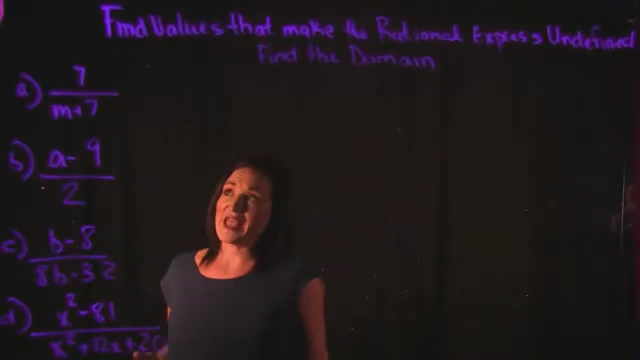 values are, and then we're going to figure out what the domain is. So, again, a rational expression is undefined when the denominator equals zero. So what we need to do to actually figure that out with all four of these? so there's only one step to this problem here as far as finding the value, and that is this Set. 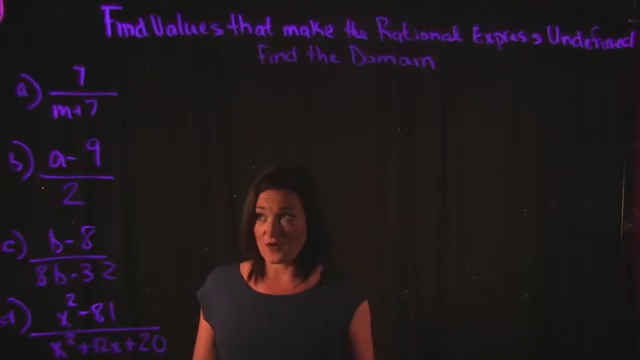 the denominator equal to zero and solve So, for example A, my denominator is m plus 7.. Literally, for this example, I don't care about the numerator. The numerators are going to have no part in this problem whatsoever. I only care. 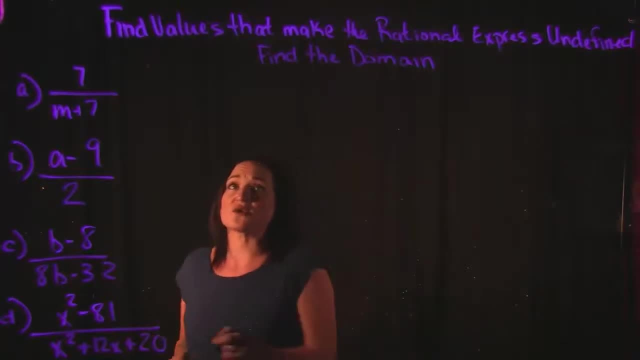 about what the denominator is specifically. what's going to make that 0.. So for A, my denominator is m plus 7.. I'm going to set that equal to 0 and solve this equation. This is a one-step equation in order to get. 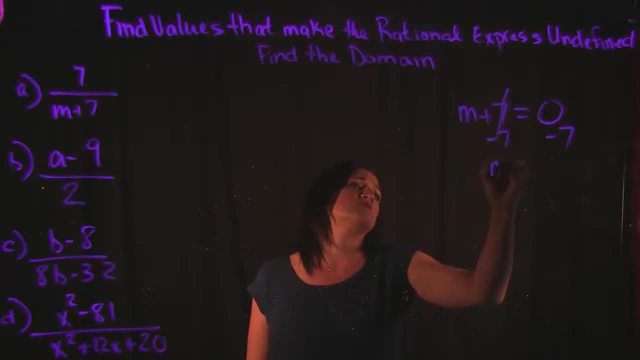 m by itself. I have to subtract 7, as long as I subtract it on both sides, And that's going to give me that m is equal to 7.. So find a value that makes a rational expression undefined. That value is negative, 7.. 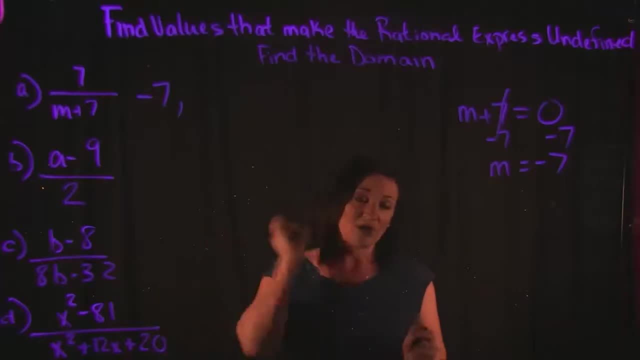 Now it also wants us to find the domain. Now, if negative 7 is what makes this undefined again, keep that in mind. negative 7 is what's going to throw this off And real quickly in your head, plug in negative 7 for m. 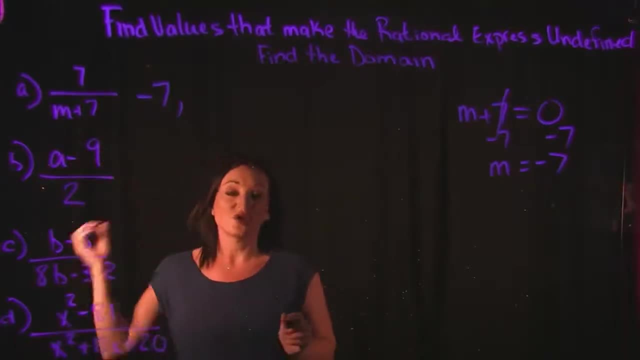 If I plug in negative 7, I get negative 7 plus 7, which is 0. That means we have 0 in the denominator and that's a big no-no. If we plug in any other number- negative 8,, negative 6,, negative 1,000,, it doesn't matter. 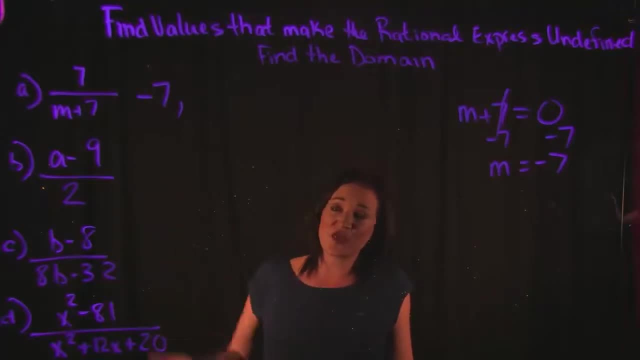 Any other number is okay. So everything except negative 7.. So one way to write the domain for that we're going to say that our domain. so if you want to say that your domain is all numbers except for negative 7, remember the domain deals with x. 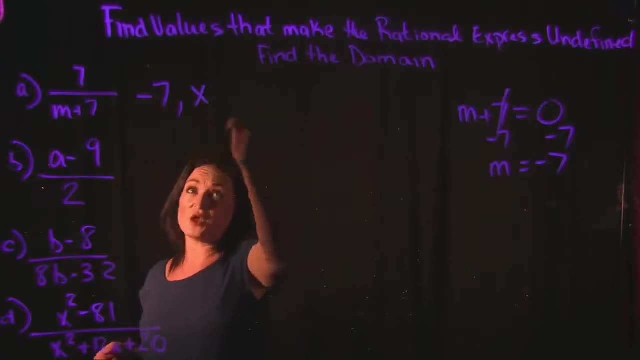 So our domain is all x values, such that x is not negative 7.. So this is a very common notation for this particular type of problem. So we said that negative 7 is what throws this problem off and our domain is everything except negative 7 is how we would write that. 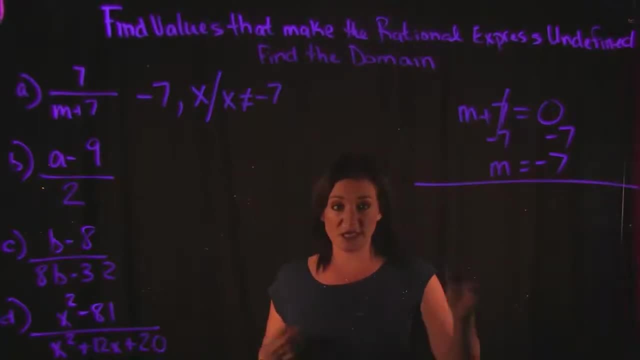 So, for example b, our denominator is 2.. So again, take your denominator, set it equal to 0, and solve. Okay, So our denominator is 2.. We're going to set that equal to 0 and solve, but I don't know about you. 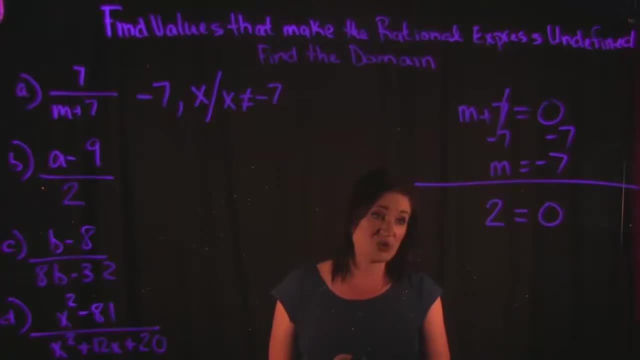 I'm taking a look at this equation and it makes no sense. It says 2 equals 0.. 2 does not equal 0. I don't even have an x or anything in this equation to solve Now. this equation itself does not make sense. 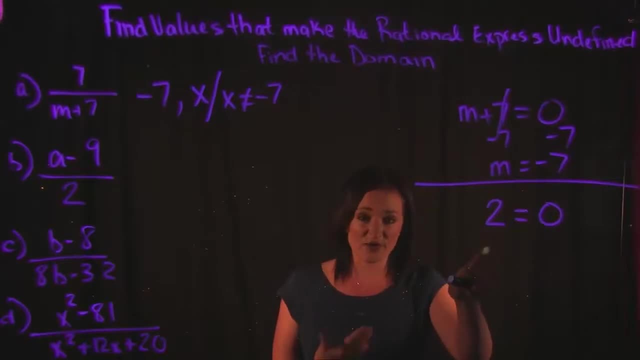 What this means is if all you have is a number for your denominator- there's literally no x- or there's no way for you to input something to make that 2 into a 0. There's no way for this to become a 0.. 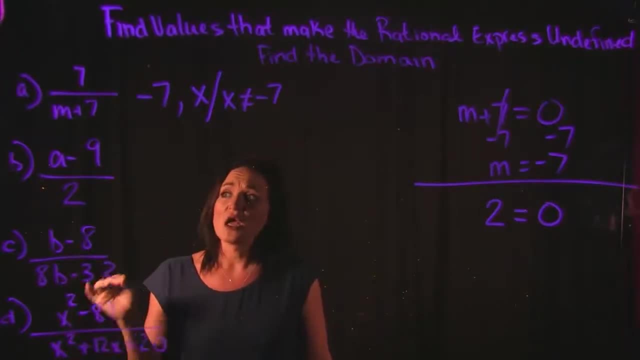 It doesn't even have an x value where we can plug something in. So if all you have is a number, like we do here, that means that there is nothing that can make this undefined. So I'm just going to say none. So that means if nothing can make it undefined, that means our domain is everything. 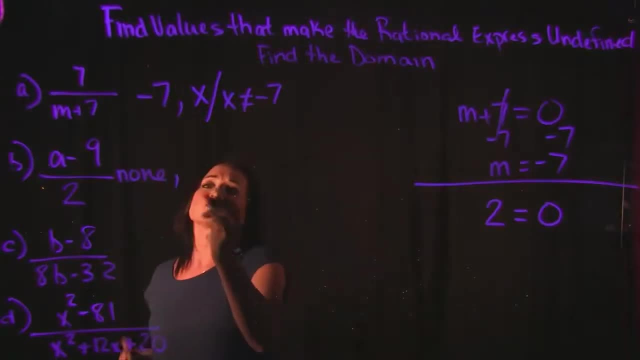 There's no exceptions, There's nothing that's going to throw it off. So that means our domain is going to be all Real numbers, It's going to be every possible number on the number line. is how that works. For example, C: our denominator is 8B minus 32.. 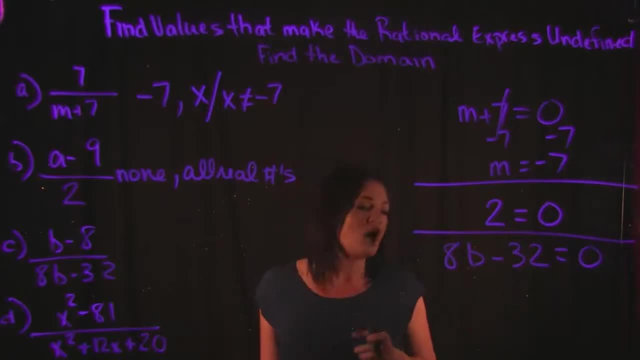 So we're going to set that equal to 0, and we're going to solve this. Now, if we're solving this equation for B, the first thing we're going to do is add 32 to both sides, which means it's going to cancel from the left. 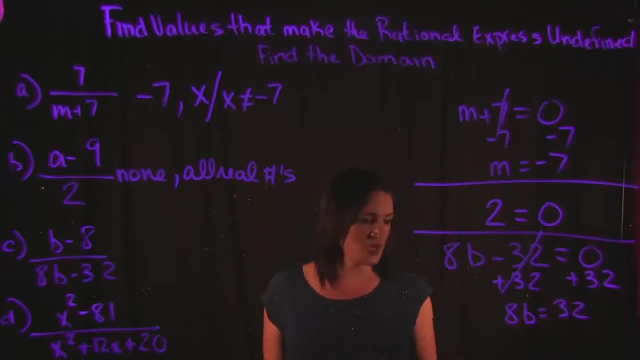 Dropping down 8B, that's going to equal to 32.. Divide out the coefficient. Remember 8B is 8 times B, so we have to do the opposite and divide. It's going to cancel on the left, giving us- and I'm not sure if you can see that- 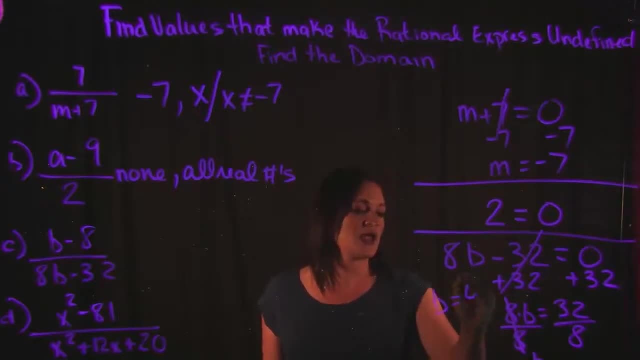 B is equal to. well, 32 divided by 8 is a 4.. So here we got. 4 is going to be the number that makes this one here undefined. That's the only number that's going to make it undefined. So our domain is all X values such that X. 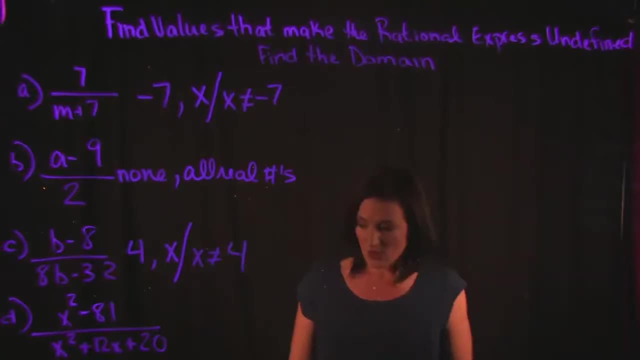 That is not 4.. That's how that works. Now, for example, D, our denominator is X squared plus 12X plus 20.. And we're going to do the same thing. We're going to take that and set it equal to 0 and solve. 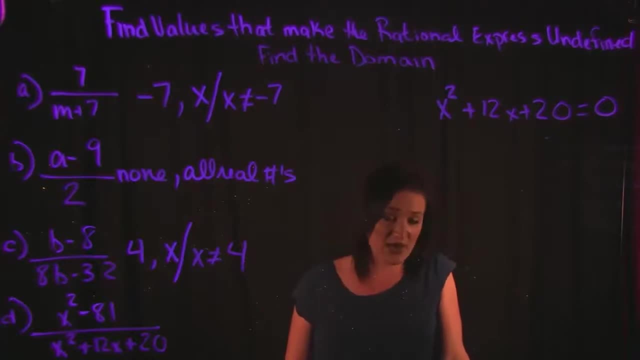 Now this one here is a little bit different, because here I have a quadratic equation. Notice this X squared term. That's going to throw this off for me a little bit here. It just means I can't solve this equation the way that I did C and A. 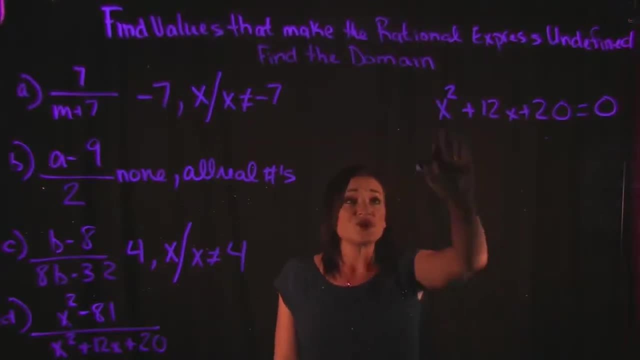 I'm going to have to solve this equation. I'm going to have to treat this a little bit differently. The way that you solve a quadratic equation. you have a few options. You can factor it, You can use a quadratic formula, You can also complete the square. 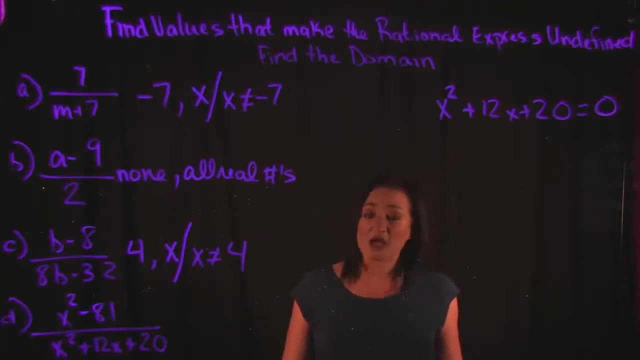 Now the easiest one to do is always check to see if it factors. That's typically your easiest technique when it comes to quadratic formulas, So that's what I'm going to go with here. So the technique that I use to factor these type of problems here is called reverse FOIL. 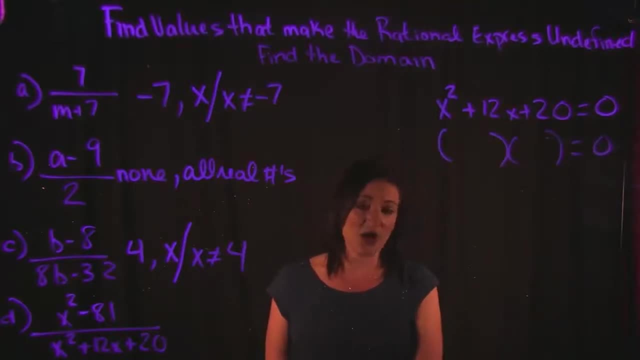 If you need to practice factoring, do look up my factoring trinomials. I have a bunch of videos and go and refresh that if you need a little bit of help with factoring. Otherwise, remember X squared. The only way you can factor X squared is an X times an X. 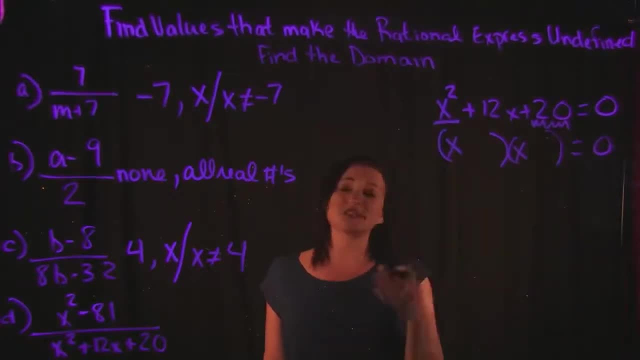 Then you jump to your last number, which is a 20, and list all the factors of 20.. So factors are 20 of 1 times 20,, 2 times 10, and 4 times 5.. What you're looking for is which one of these combinations- combination 1, 2, or 3,? 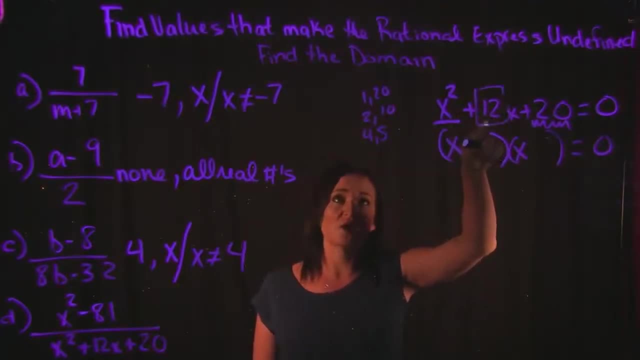 adds or subtracts To get your middle number in your equation, So like 1 plus 20,, 20 minus 1.. 2 plus 10, 10 minus 2.. 4 plus 5,, 5 minus 4.. 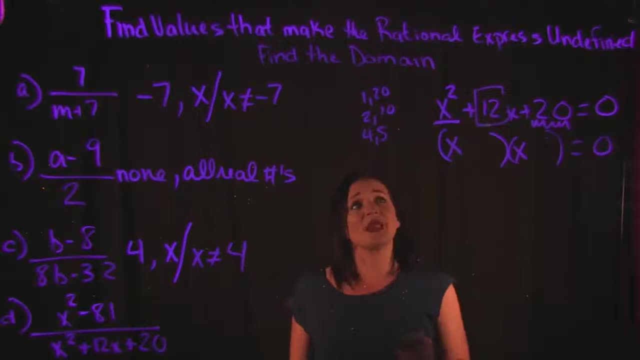 You're looking to get the number 12.. Out of all those combinations, the only way to get 12 is using 2 and 10.. 2 plus 10 is 12.. So that means these are the two numbers I want to use. 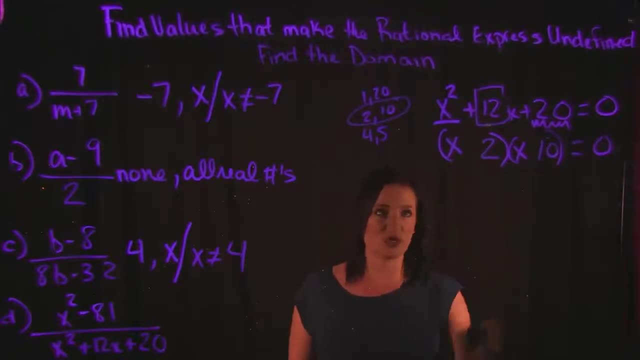 So I'm going to put in 2, and I'm going to put in 10.. Doesn't matter which one. You can say 2 and 10.. You can say 10 and 2. It doesn't matter. Then you look at your signs. 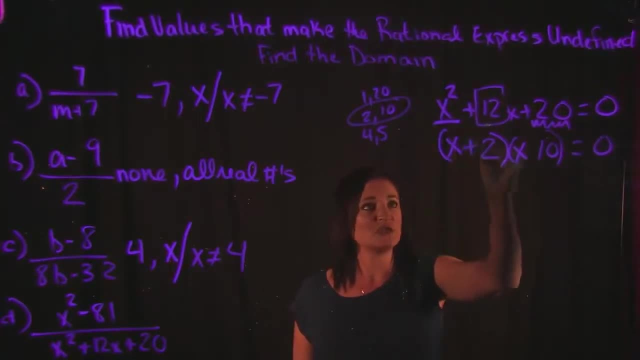 Everything in my trinomial appears positive, which means my signs inside here are also going to be positive. Then I have the problem factored. Now we need to solve it. Remember that once you have it factored, what you do after this point is you split your two factors up. 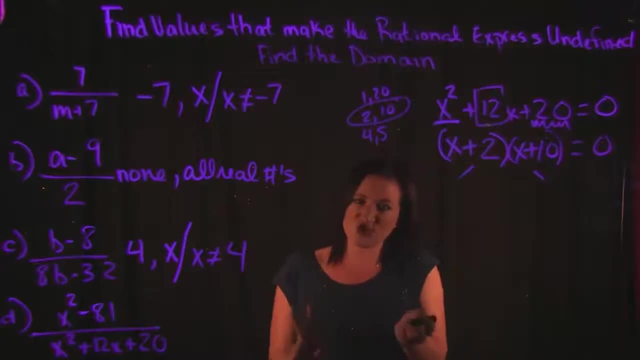 and you set them each equal to 0 to solve. So you create too many equations. So that's going to look like x plus 2 is equal to 0.. x plus 10 is equal to 0. And solve both. So the first one here I would subtract 2 on both sides to get x is equal to negative 2.. 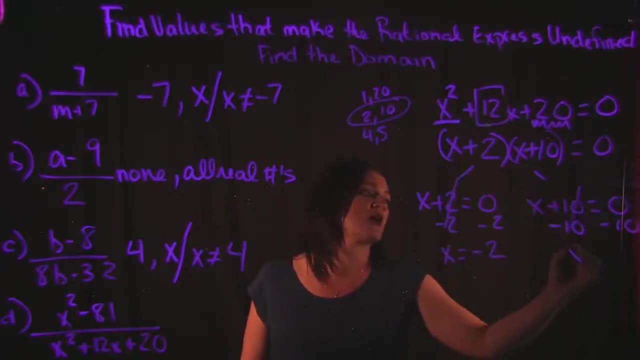 Over here. I'm going to subtract 10 on both sides. getting x is equal to negative 10.. So that means negative 2 and negative 10 are both values that make my expression undefined. So I'm going to say negative 2 and negative 10..